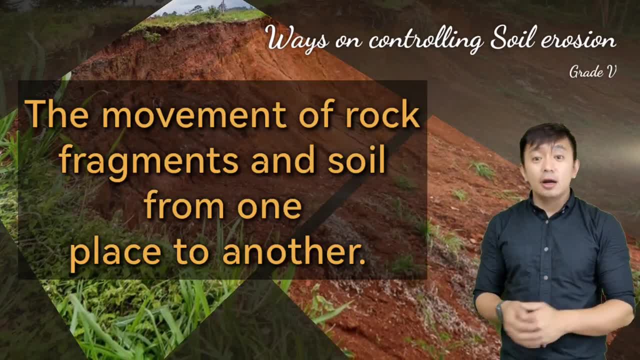 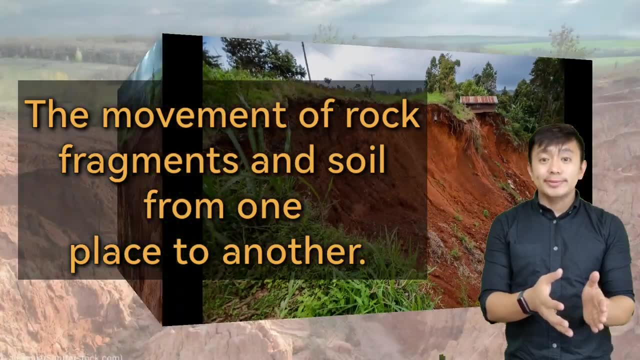 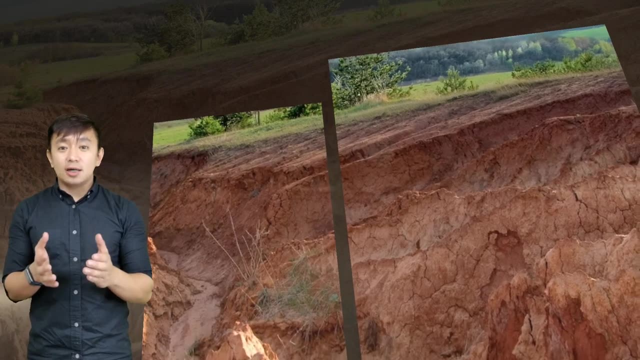 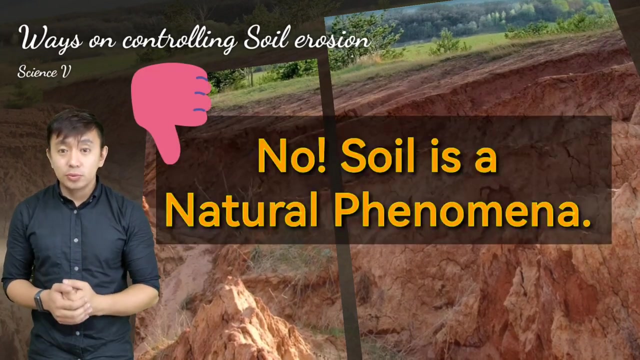 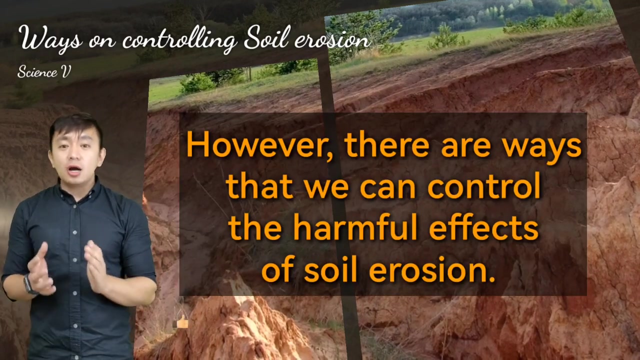 If we say erosion, this is the process wherein rock fragments and soil moves from one place to another. The next question is that: can we prevent soil erosion? The answer is no. Soil erosion is a natural phenomenon in the environment. However, there are ways on. how are we going to lesson? 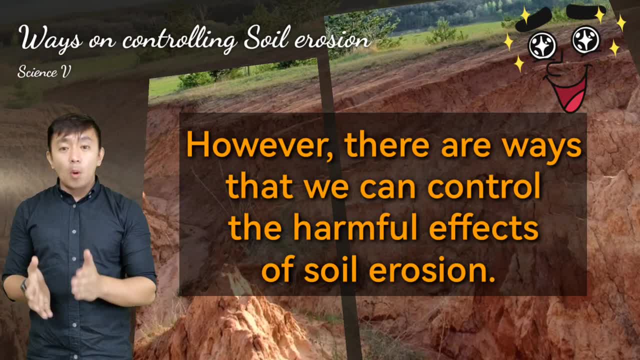 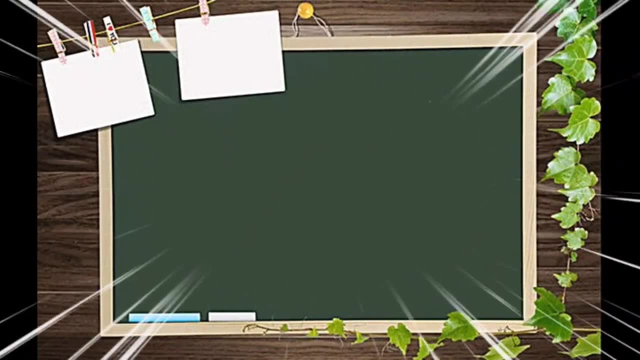 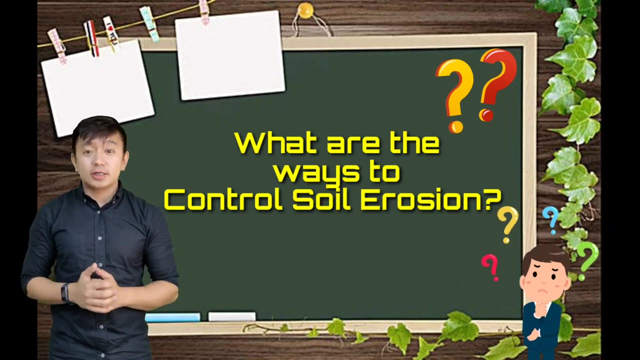 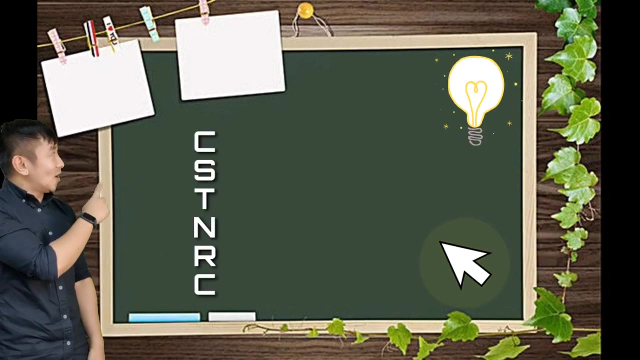 And prevent its harmful effects, both in the landforms and abiotic factors. So what are the different ways on? how are we going to control the harmful effects of soil erosion? Again, remember this acronym: CESNAR-C. C stands for Contour Flowing. 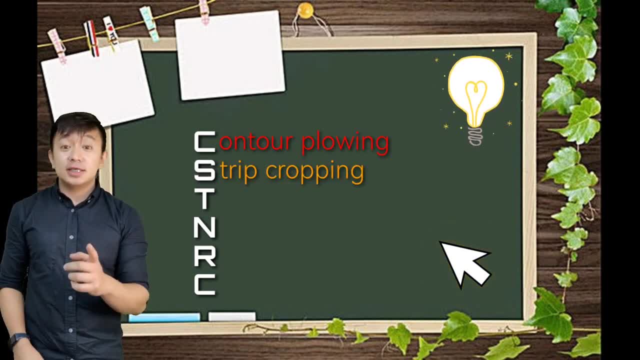 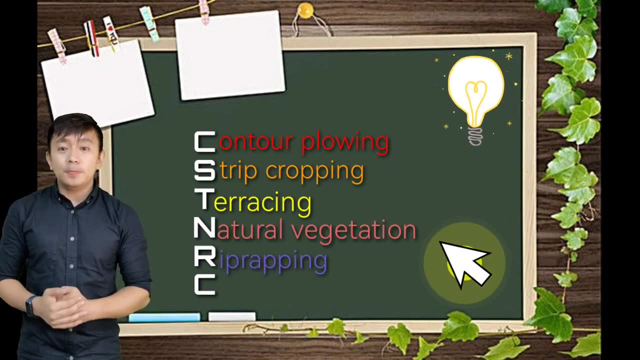 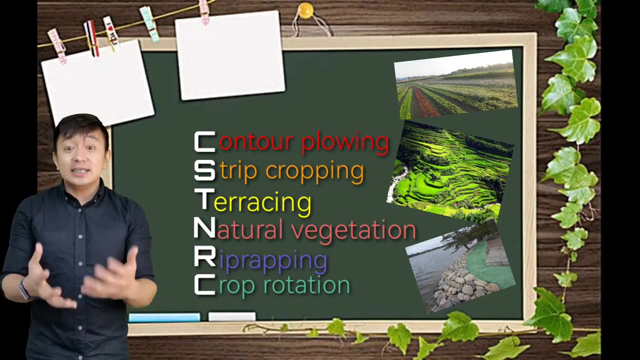 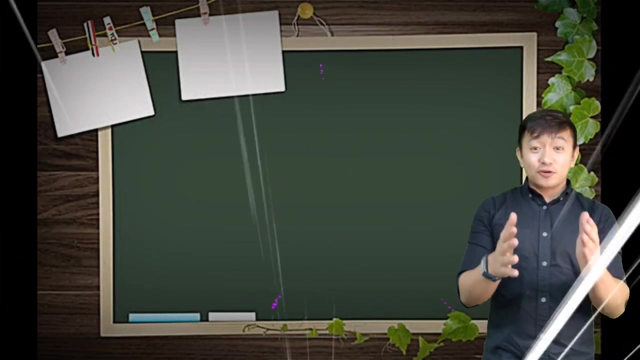 S- strip cropping, T- terracing, N- natural vegetation, R- rip cropping And C- you have your crop rotation. So let's describe these six ways on: how are we going to prevent soil erosion? The first method in controlling now soil erosion, we call this one as control. 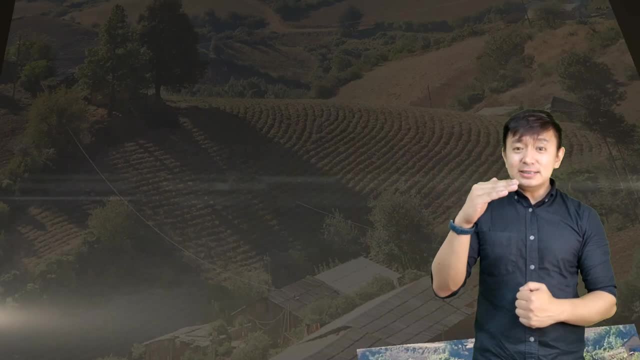 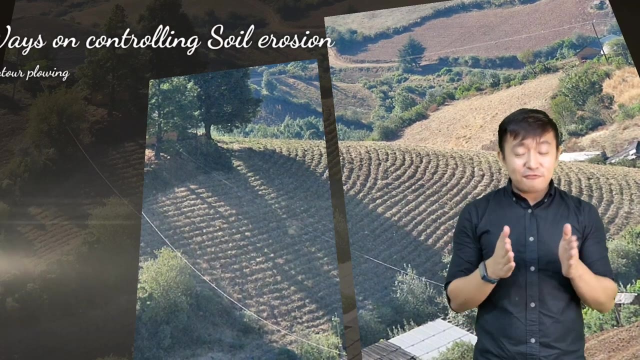 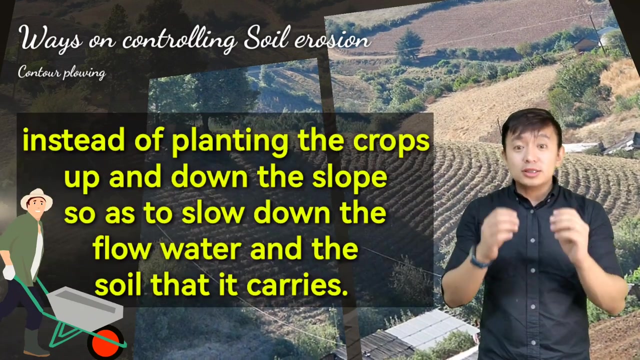 And the second method in controlling, now, soil erosion. we call this one as a contour ploughing. Since erosion takes place easily in the soil, what will the farmers do? They follow the curves of the mountain. When they follow the curves of the mountain, we call this technique as contour ploughing. 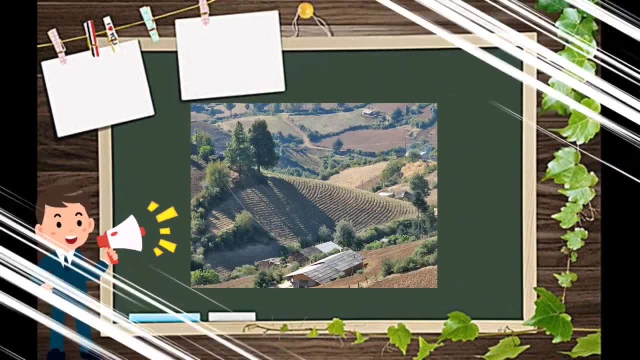 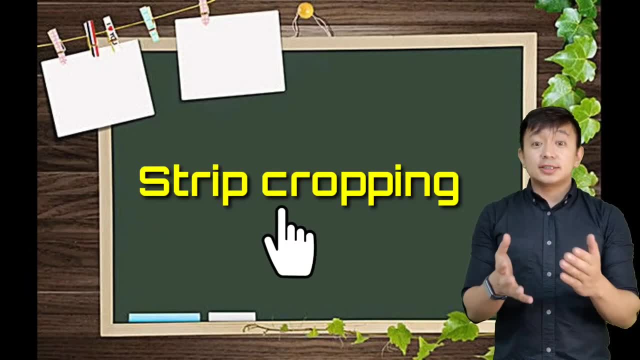 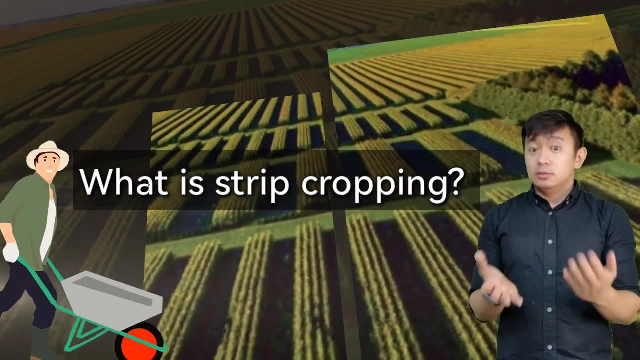 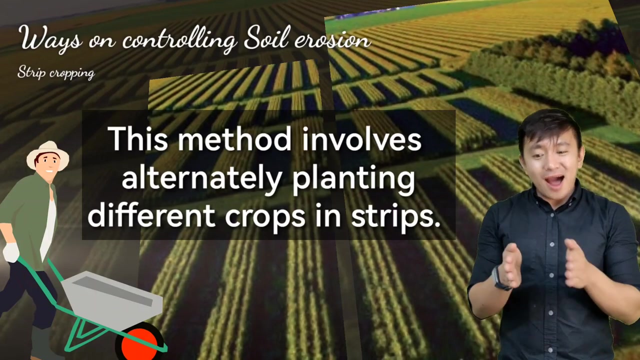 The second method in controlling now, soil erosion is called contour ploughing. The second method in controlling nail soil erosion, we call this one as strip cropping. Now what is the difference between strip cropping from that of a contour flowway? In a strip cropping, you are actually planting alternately crops. in a strip. 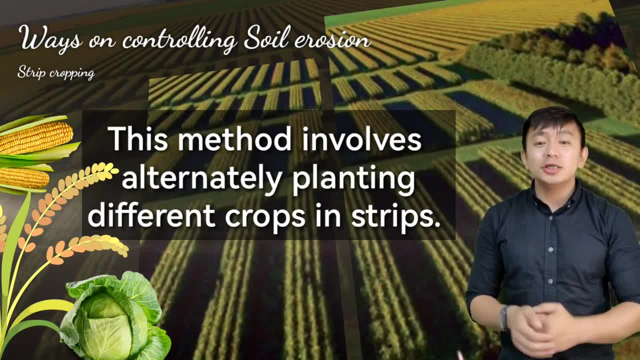 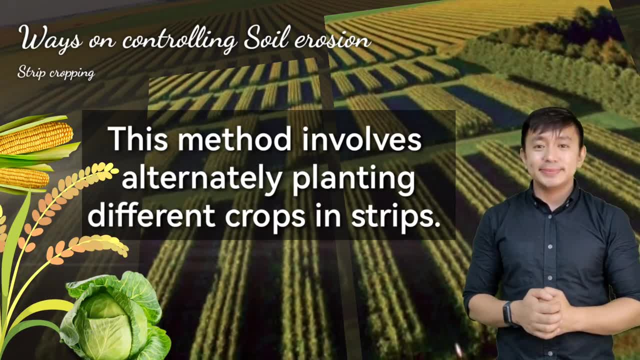 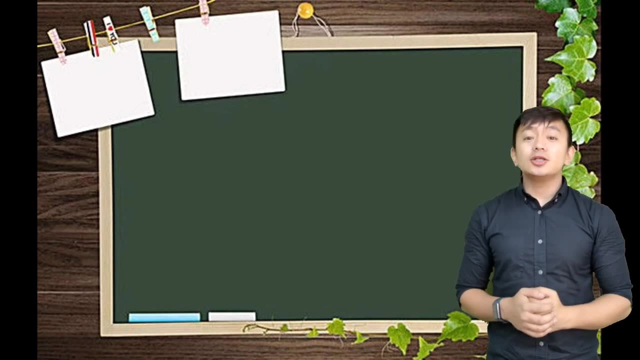 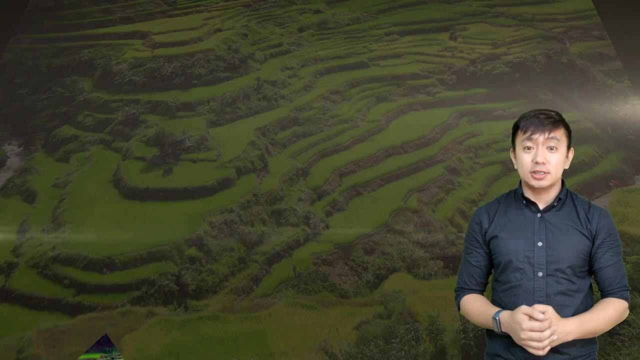 And in this technique you are actually controlling the flow of water. Your key term there is, alternately, The third method in controlling nail soil erosion: you have terracing. Have you ever been to Banaue Rice Terraces Or do you have a picture of it? 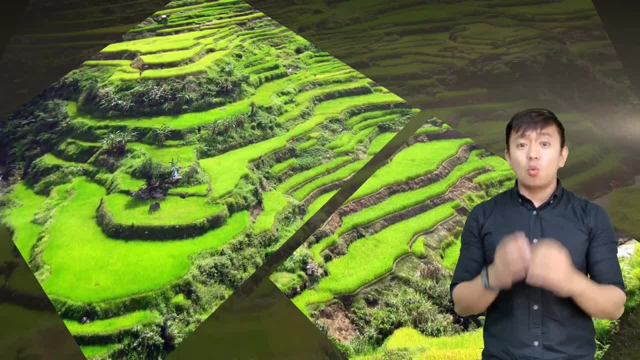 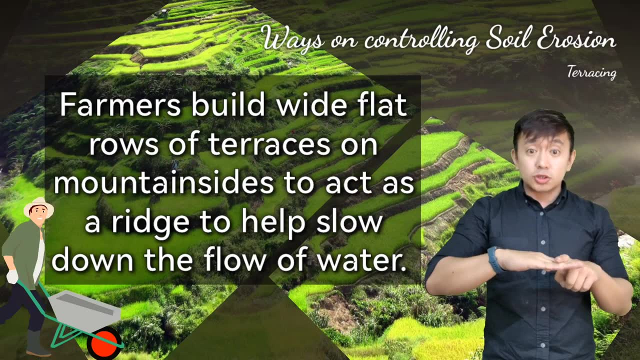 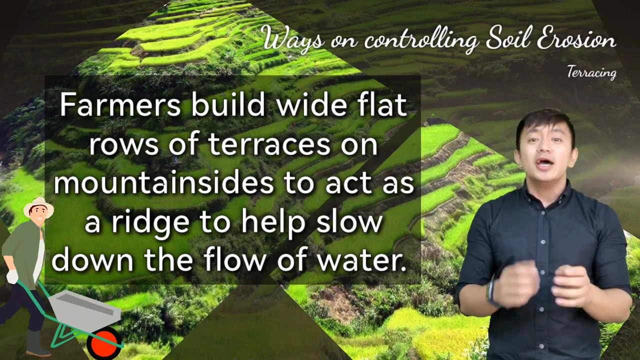 That is a good example now of terracing. So what do the farmers do? The farmers are actually building a wide, flat rocks wherein it serves as a ridge to control the flow of water. By doing such, they are actually controlling the harmful effect of soil erosion. 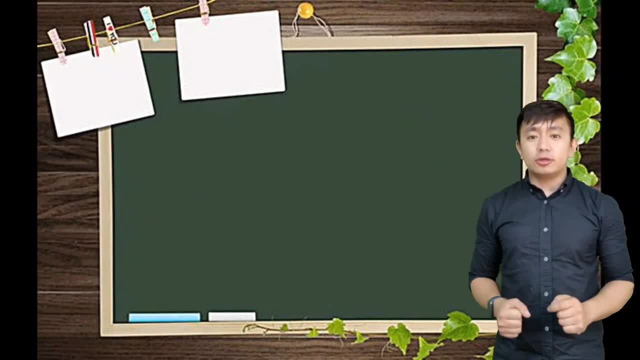 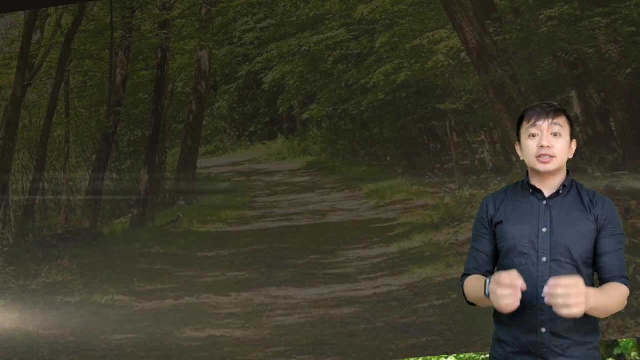 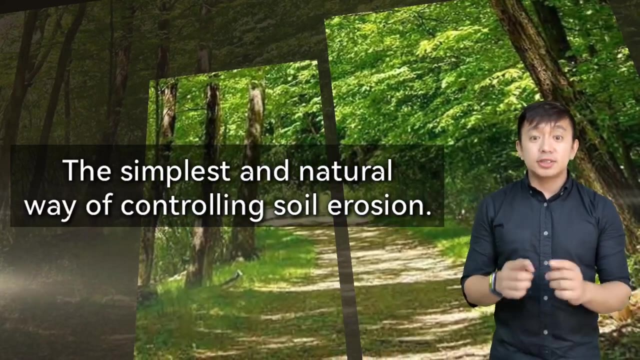 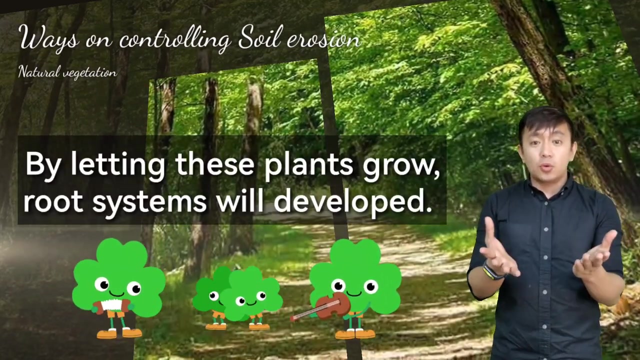 So another way of controlling soil erosion is through They grow natural vegetation. Natural vegetation actually is considered as the simplest form of controlling soil erosion. But how are we going to do that? We allow trees and plants to grow naturally. Therefore, there is the development of root system. 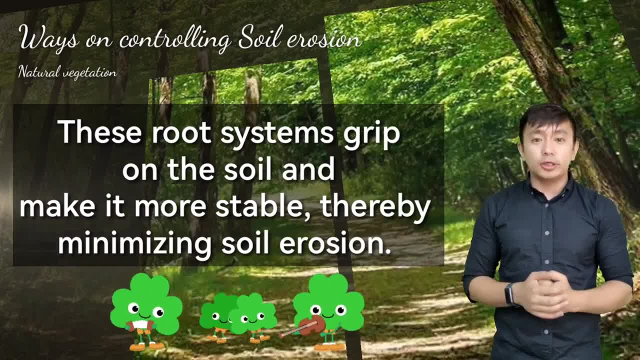 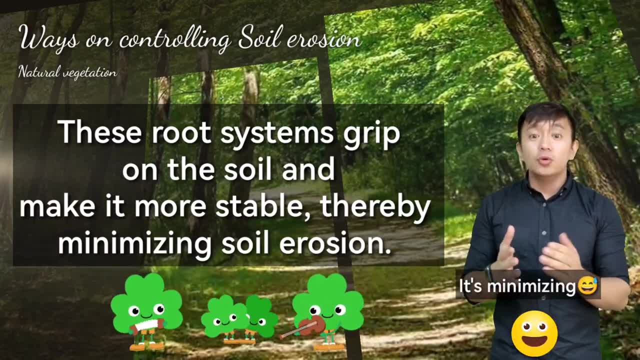 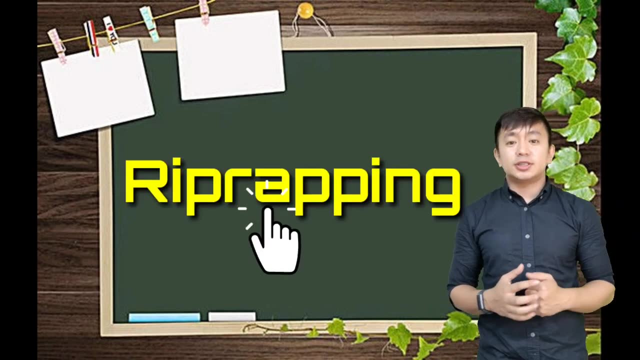 And this root system grips on the soil, Which allows it to be more stable and it maximizes now the flow of erosion. Another way of controlling soil erosion is through rip-ropping. So how do we do rip-ropping? It's very simple. 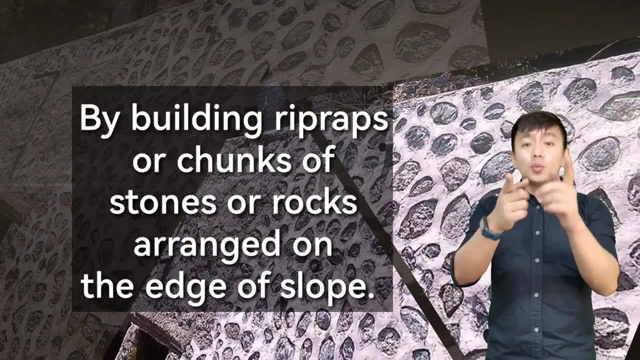 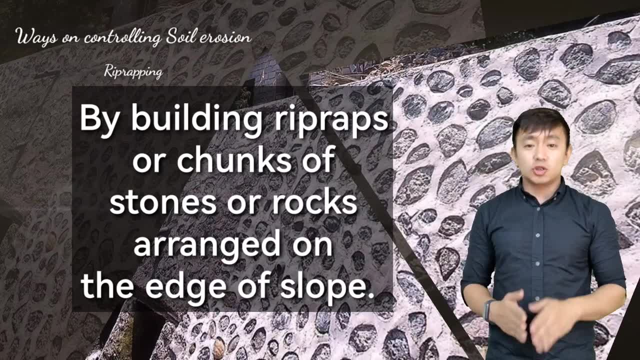 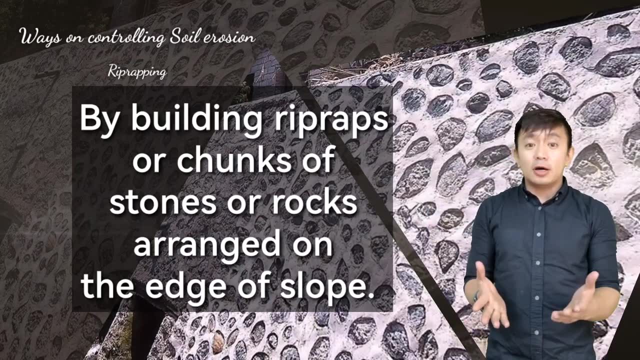 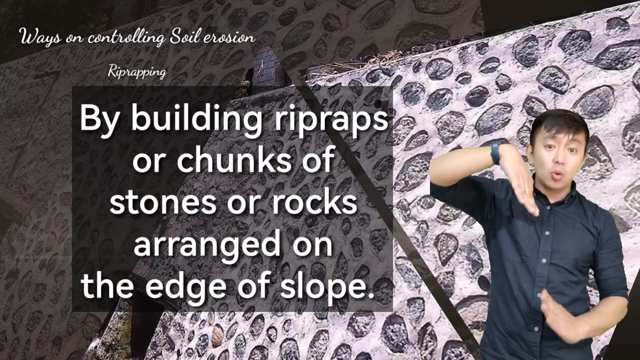 By building chunks of rocks or stones, we are building foundation, But actually it's not only building foundation. It allows us. It allows us to control the movement of the soil going down. Where do you usually find the rip-rops? We usually find them along seashores, shorelines or just below a slope. 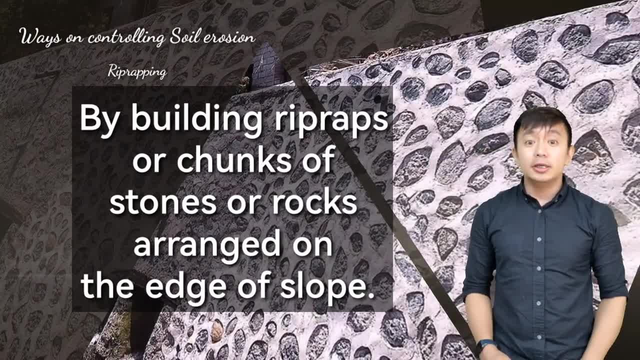 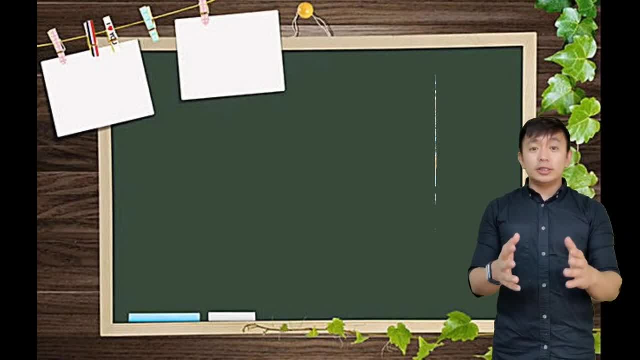 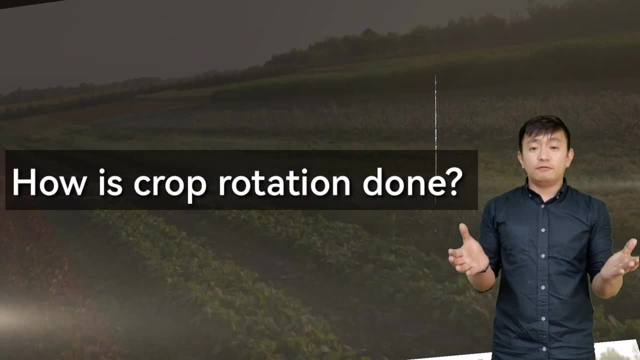 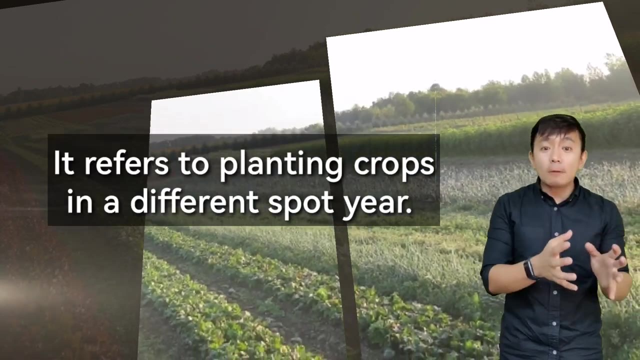 In this manner, we are actually controlling soil erosion. So the last method in controlling now soil erosion is through Through, Through crop rotation. So what do we usually do if we are talking about crop rotation? In a crop rotation, it refers to planting crops in a year.